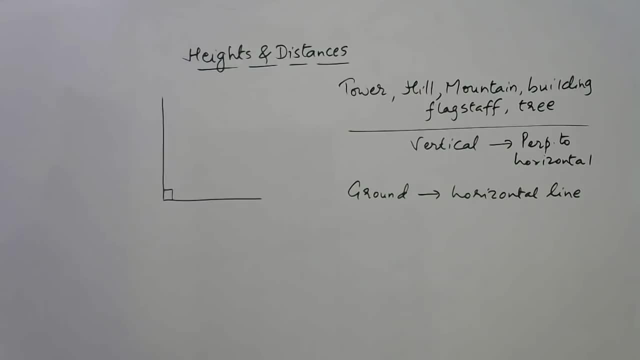 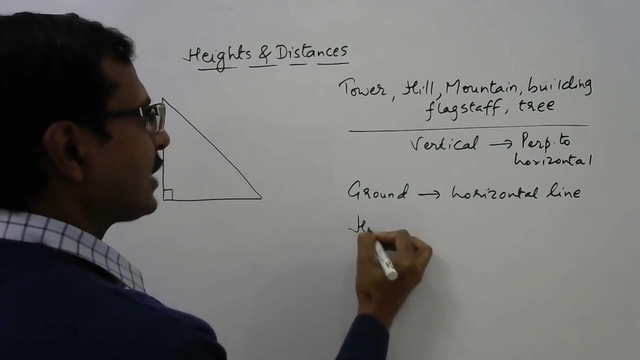 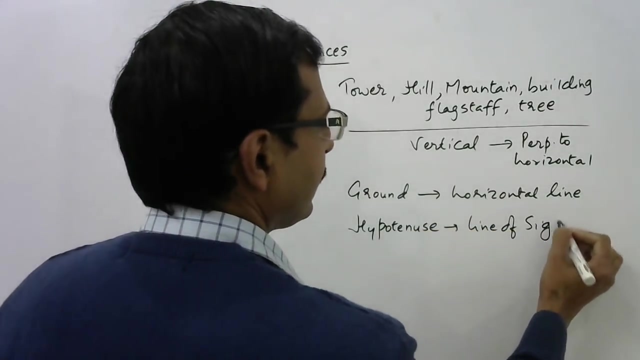 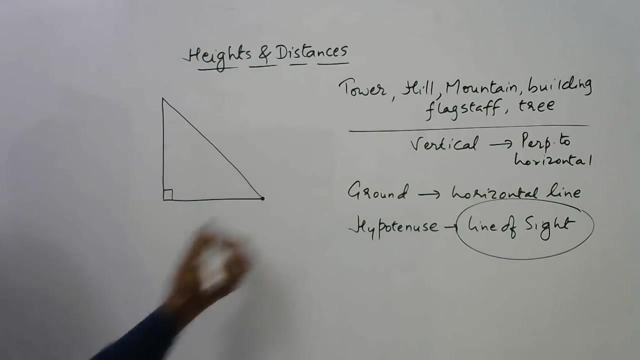 triangle: One is the vertical line and the second one is the ground level. Now come to the third side, which is the hypotenuse. Now, this side, hypotenuse, is actually called the line of sight, And line of sight is the line on which we see. Now suppose a person is standing here and he is looking at the 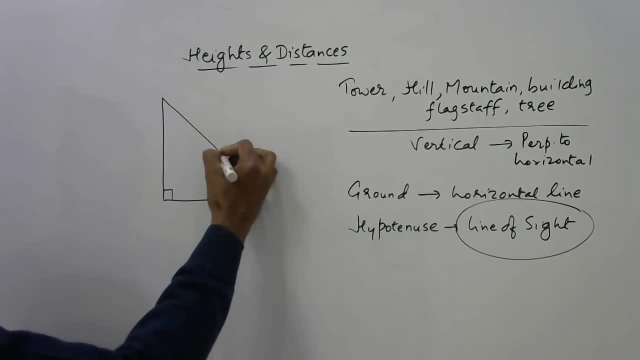 top of this vertical object, Then this is called the line of sight. Or it can be the other way round: The person is standing on the top of this building and watching something on the ground, So this can be the object and this can be the observer. 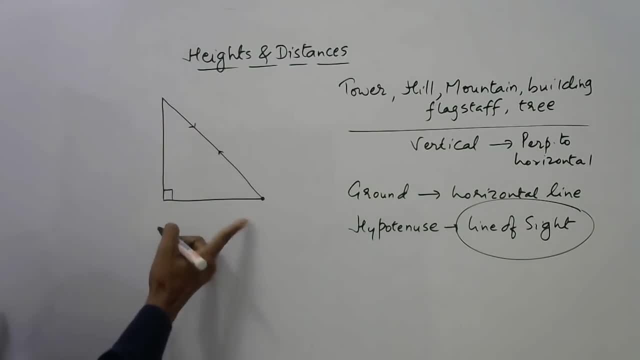 So if the observer is here, then the line of sight is like this: If the observer is here, then the line of sight is like this: So we have the line of sight represented by the hypotenuse, The horizontal line which is the ground level. So this is the horizontal line And the horizontal line which is the 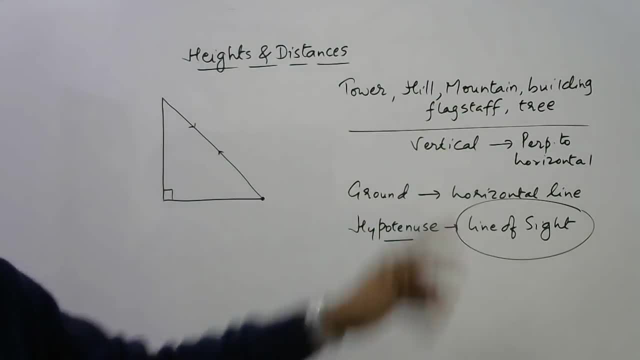 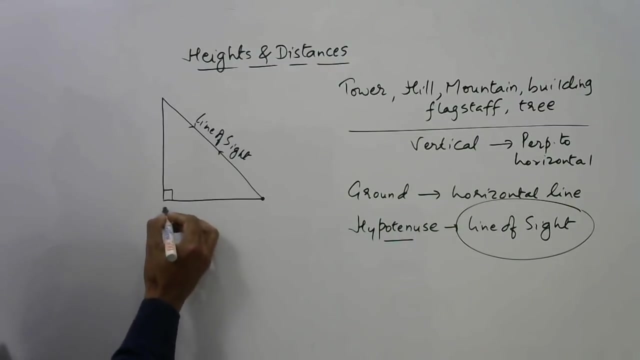 ground And the vertical line which is the tower hill mountain building or the flag staff. So we have three sides of a right angle triangle here Now, this line of sight and the horizontal, the angle which these two lines are making. 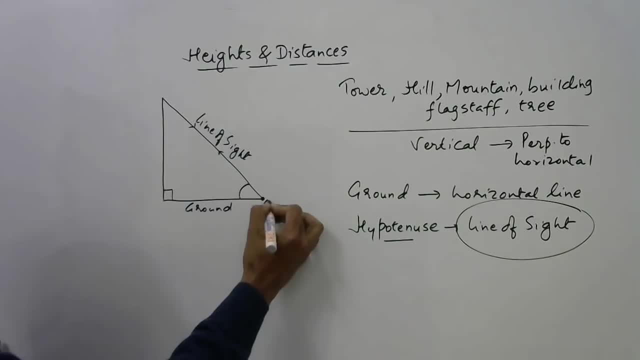 the ground and the line of sight, And this point is the observer. This angle, acute angle, is represented by theta And this angle is known as angle of elevation. So whenever the observer is on the ground and he is watching something above him, then the angle which the line of sight makes with the ground is known as the angle. 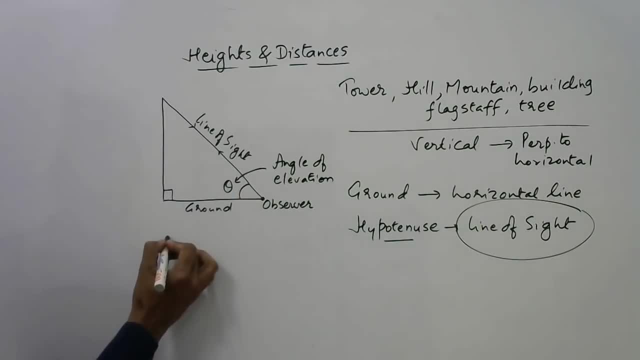 of elevation. Now take the other case. Now this is the vertical object, This is the ground And this is the vertical object, And this is the angle, And this is the vertical object. hypotenuse: Now the observer is here at the top of this tower and this is the line of sight.